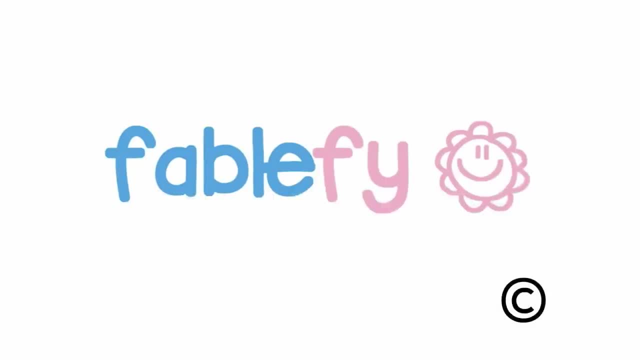 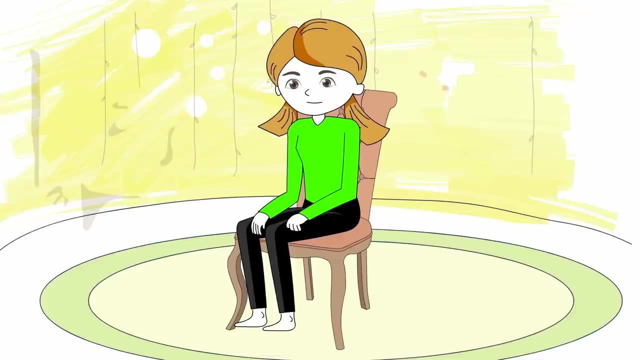 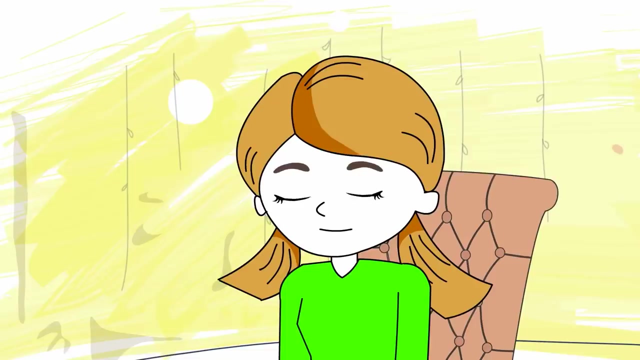 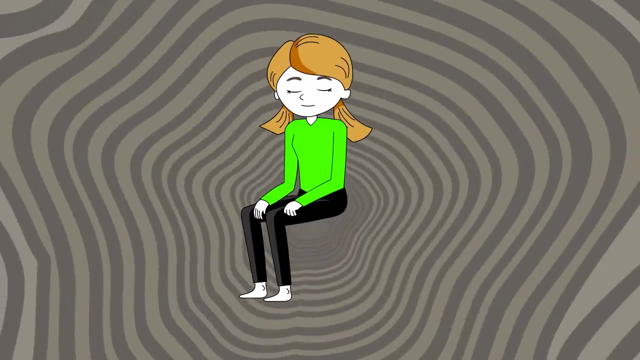 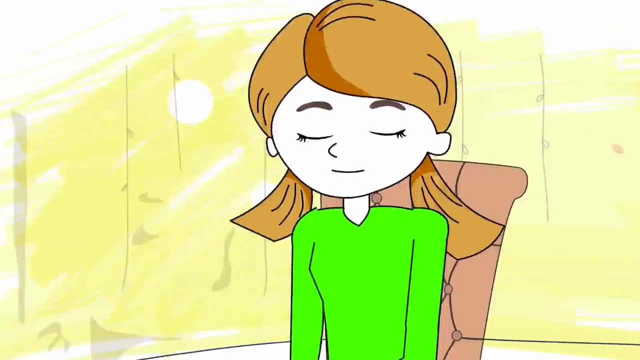 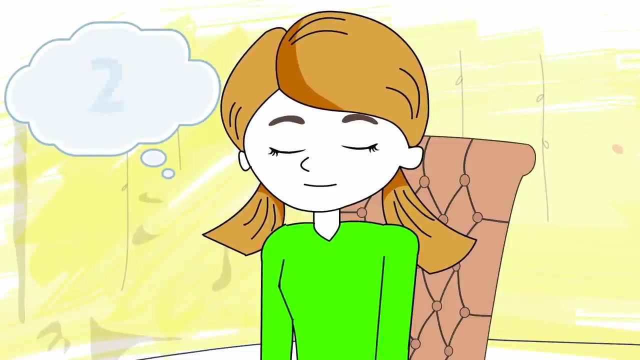 Fly with Abel and Fi. Body scan meditation. Sit in a comfortable position and bring attention to your body. Close your eyes if that's comfortable for you. You can notice your body, seated wherever you are feeling the weight of your body- on the chair or on the floor. Take a few deep breaths, Breathe in through your nose. One, two, three, four. 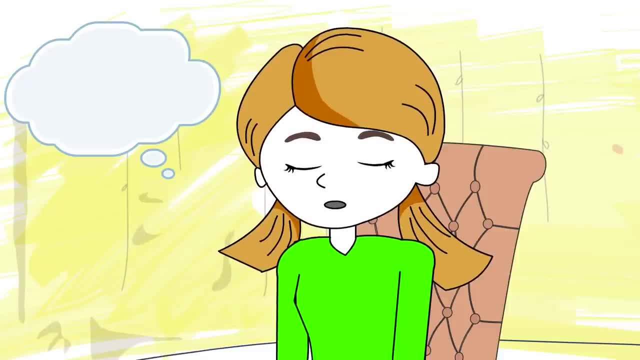 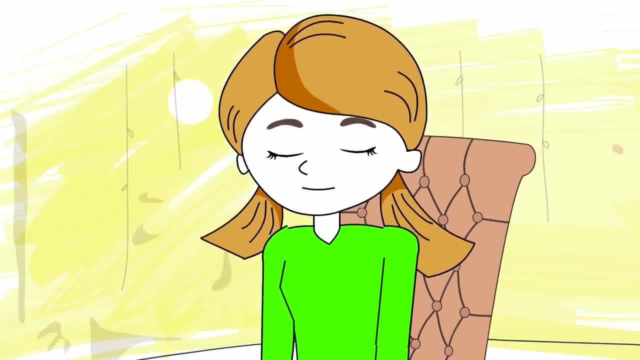 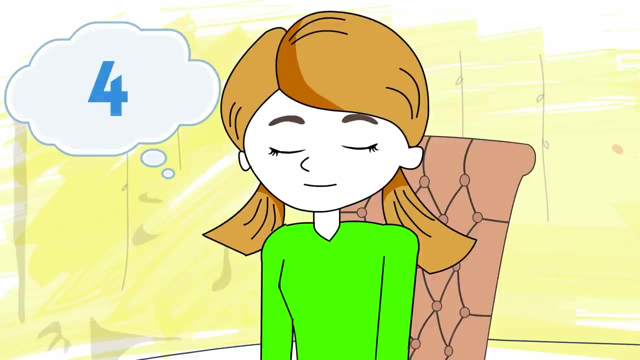 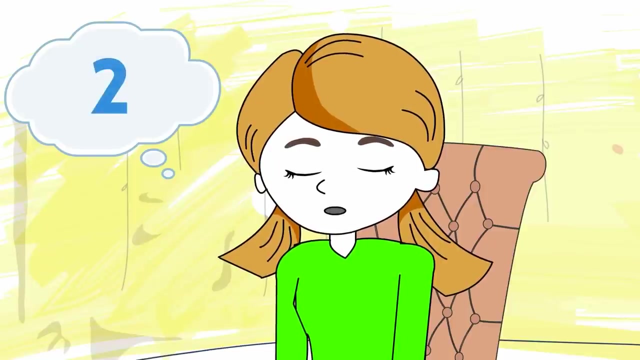 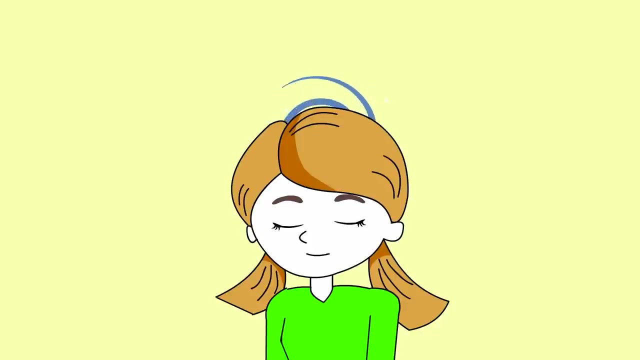 Breathe out through your mouth Four, three, two, One. Breathe in through your nose: One, two, three, four. Breathe out through your mouth Four, three, two, one. Now bring your attention to the top of your head. Sense this area. What do you feel? Stillness. 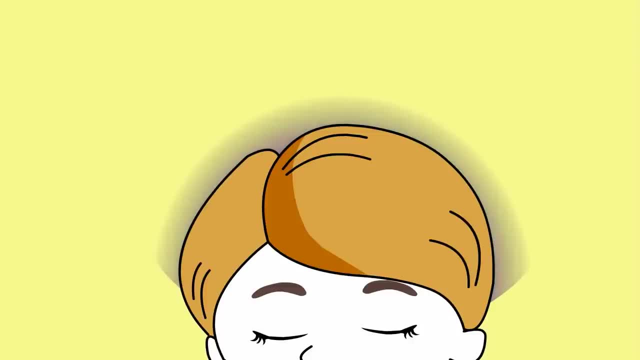 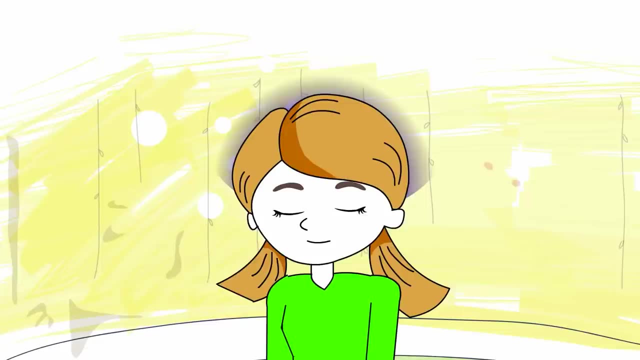 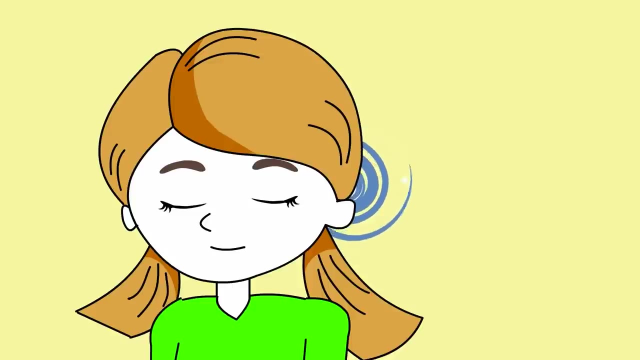 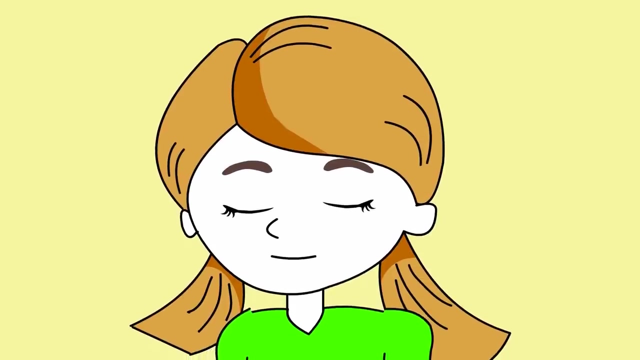 or a feeling running through your hair. Breathe And, as you breathe, relax the top of your head. Continue to breathe and move your attention to the side of your head, in your ears. What do you sense? Do you hear anything? Now bring your attention to the neck and throat. Let them be soft. 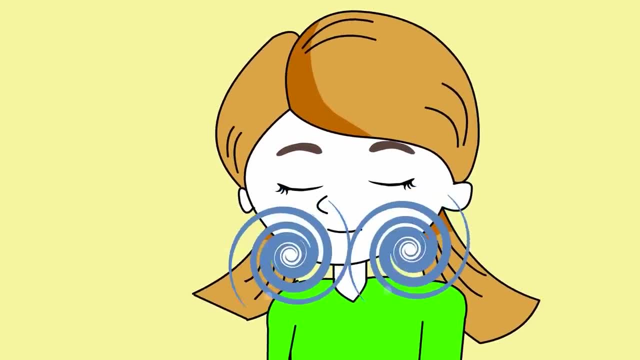 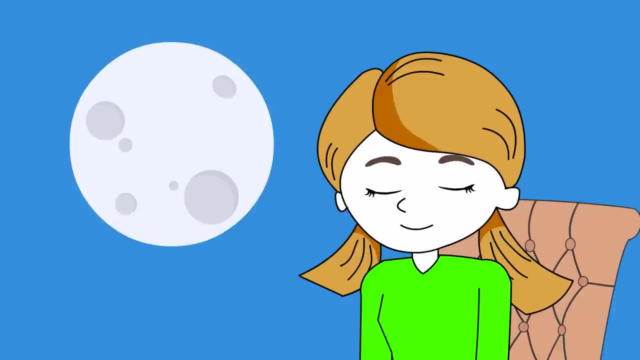 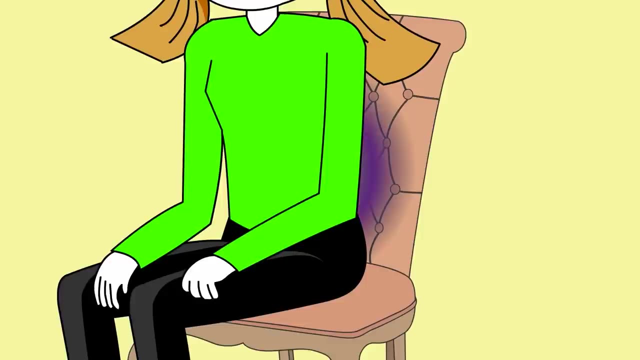 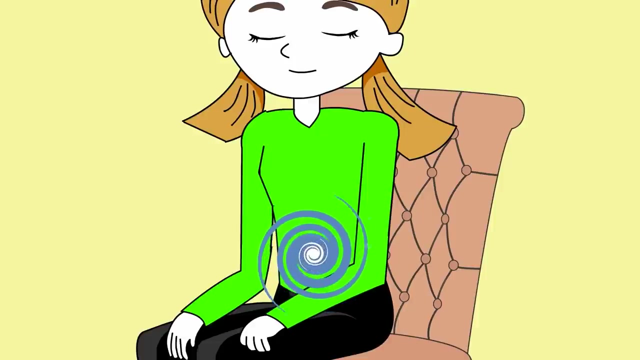 Relax. Soften your jaw. Let your face and facial muscles be soft. Smile softly and gently. Notice your back against the chair. Bring your attention into your stomach area. If your stomach is tense or tight, let it soften. Take a breath, Feel pressurefish backwards and back. Let your natural stress get to your heart. Relax your shoulders and olhos pushed into this muscle. Feel tension. Relax your shoulders and elbows. sprained sleeve. Open your body�